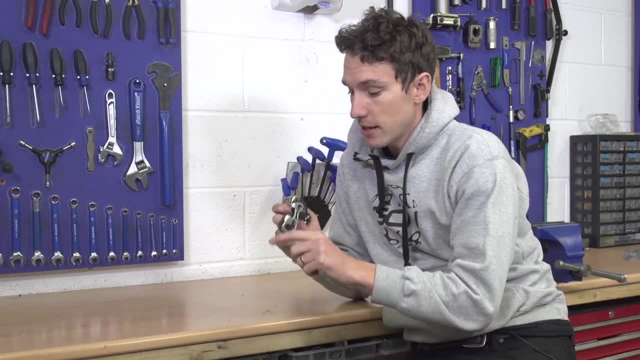 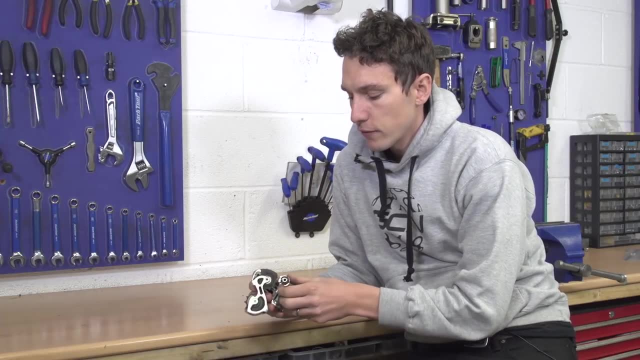 The reason that it has broken, as you can see, partly the jockey wheels are worn out, but that's easy to replace. We have a video already on that subject. This one is suffering from two frozen pivots. The first one that allows the whole derailleur to pivot back. 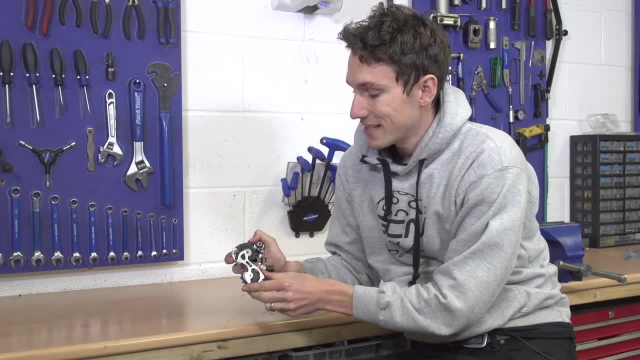 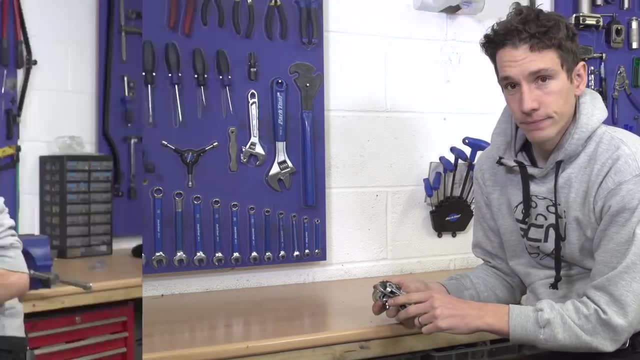 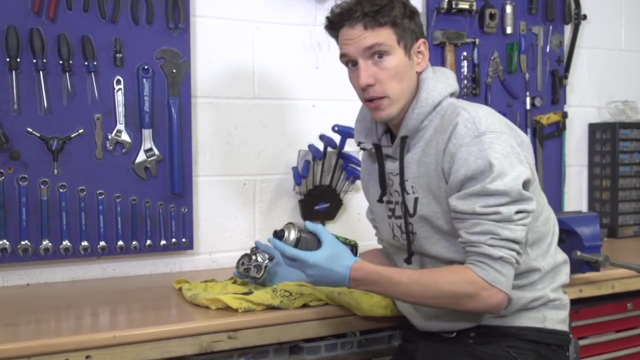 on your frame, Then the second one, which allows the jockey wheels to actually tension, the frame has, you can see, completely seized up. We'll start very simply by giving it a thorough clean Using a solubilizer That, basically, is just going to make it more pleasant to work on, if nothing else. 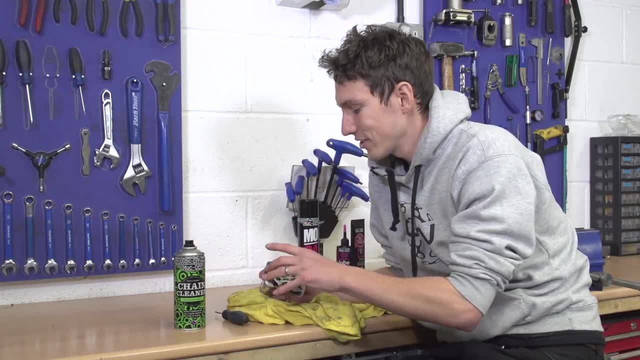 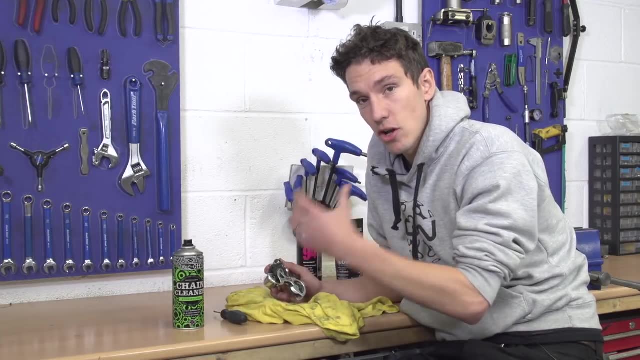 If either pivot freezes, like with this one, generally it's just a case of taking them apart and then really thoroughly degreasing them and regreasing them, because basically they just get so gunked up and slightly corroded. That is what we're going to do now. It is. 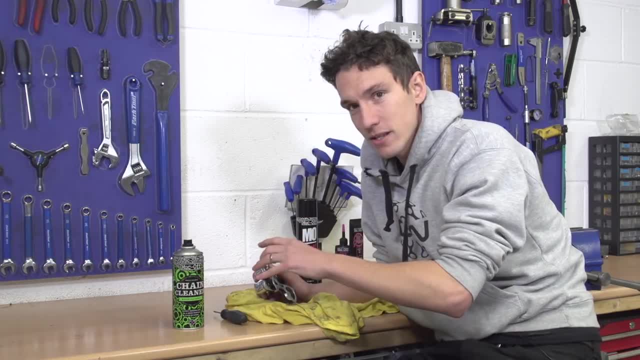 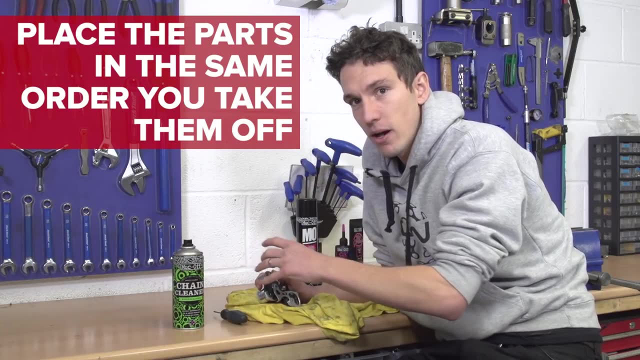 a reasonably complex job. There are an awful lot of small parts in here, parts that need to be reassembled in the correct order. Proceed with a little bit of caution and remember that anything that you do take apart, just keep a record of the order in which it comes. 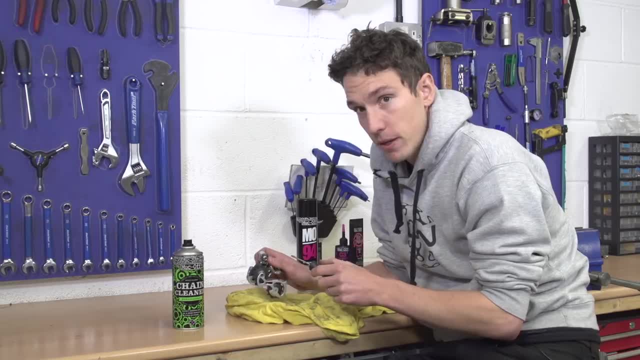 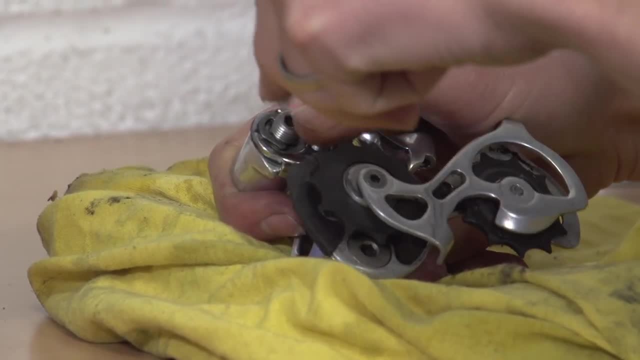 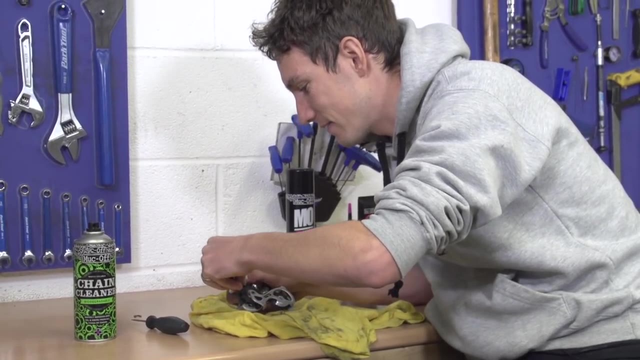 apart in First up, let's do the top pivot bolt. We need to remove this little circlip first of all. There is, as you can probably remember, quite a powerful spring in here. It is starting to unwind, Okay. 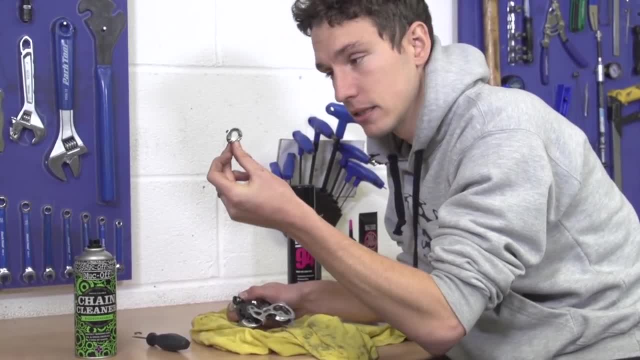 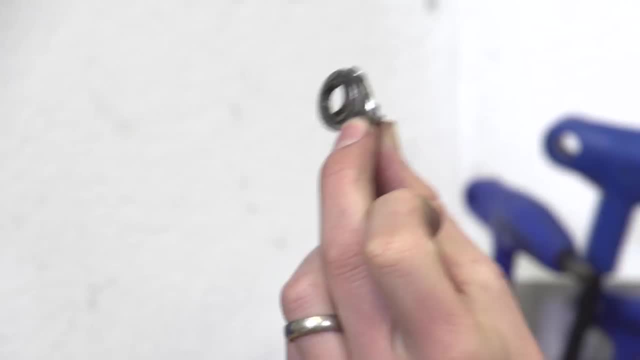 First thing that comes out of this is the spring. This is the spring. This is the spring. The first thing that comes off is that: so our B-tension adjustment plate. On the other side of it, you'll see there's a little hole there. That is the hole that our spring goes. 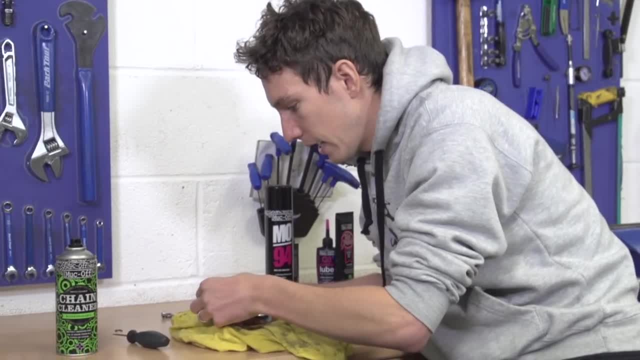 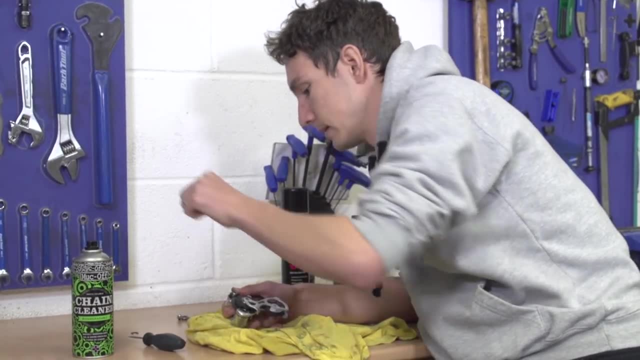 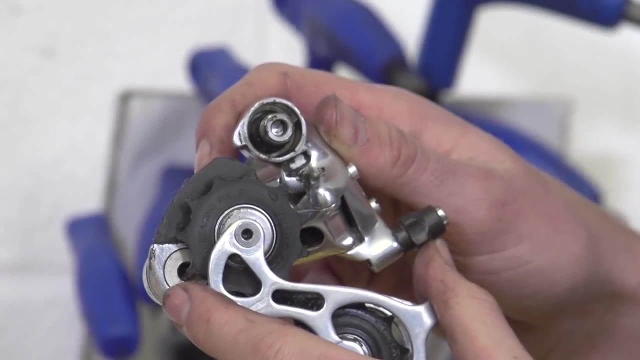 into. so remember that, Pop that there. Then we've got a seal which has done its job admirably for 14 years. Then we've got a spring. There we go. It's as simple as that in there. The. The second one is a little bit more complex perhaps. 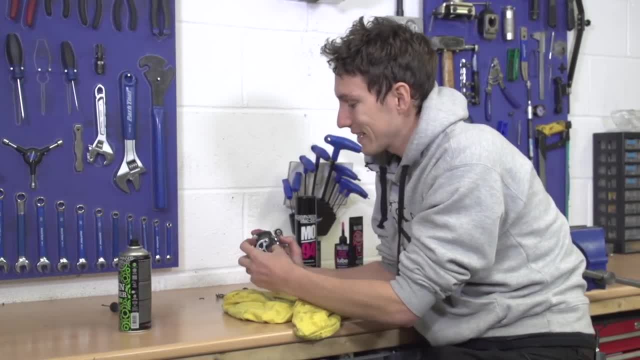 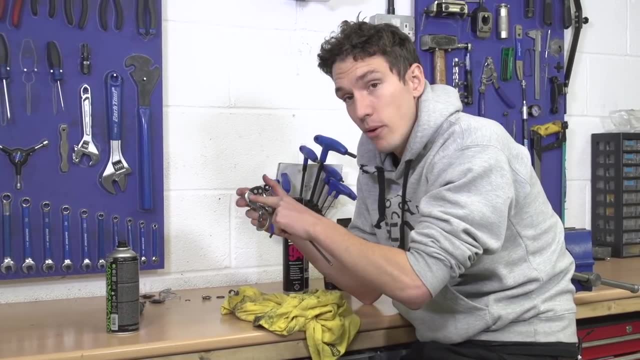 and to start with, we're gonna need to take off the jockey wheels so that we can actually get access to that bolt there To remove this lower pivot. then we need a five mil Allen key and we just need to unscrew. 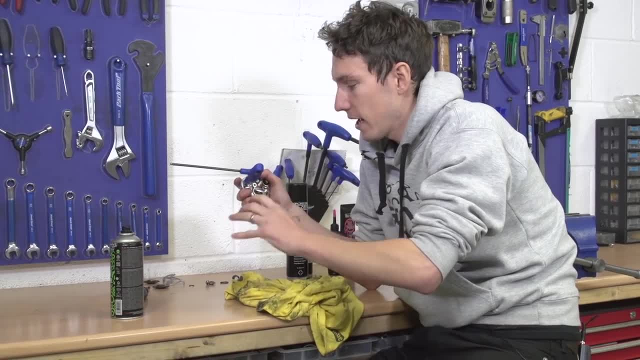 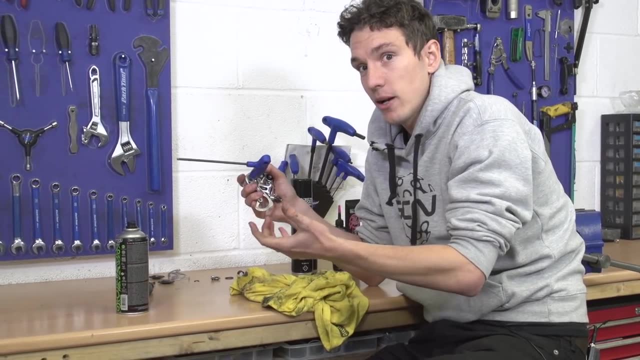 At this point you really, really need to be careful, because the derailleur cage will start to unwind and we need to remember which way it unwinds so that then, when it comes to putting the tension back in, we do it the right way. 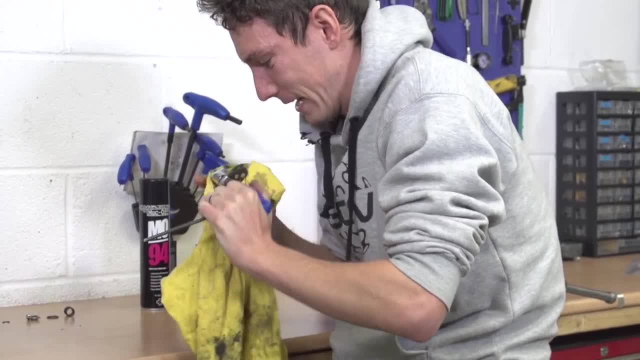 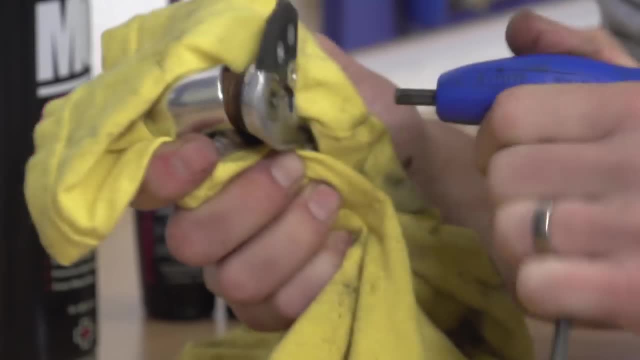 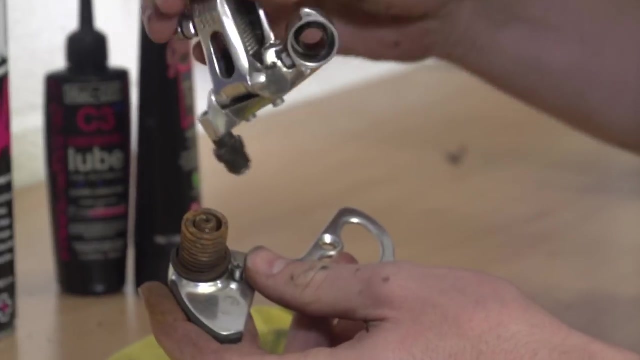 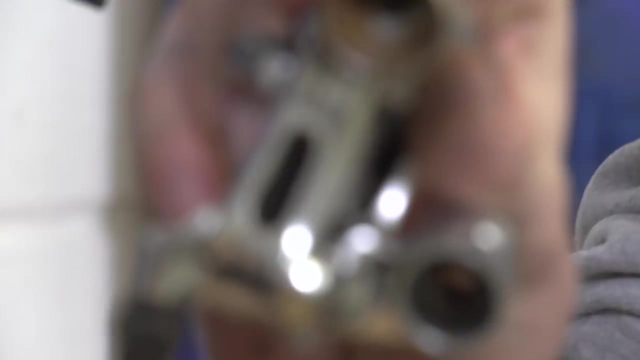 There it goes. I don't have any biceps Right. come on then, Ready. oh, there we go. Oh man, look at that. Yeah, that's probably why it wasn't moving very well. Can you see that? 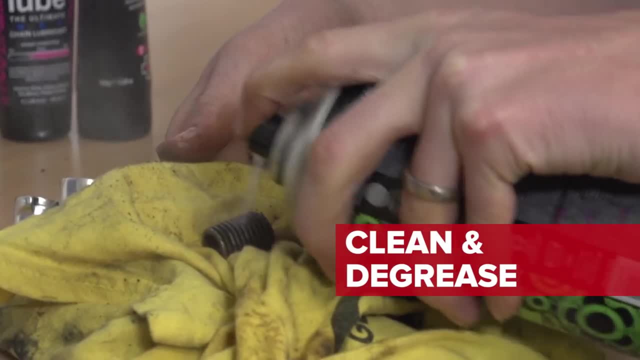 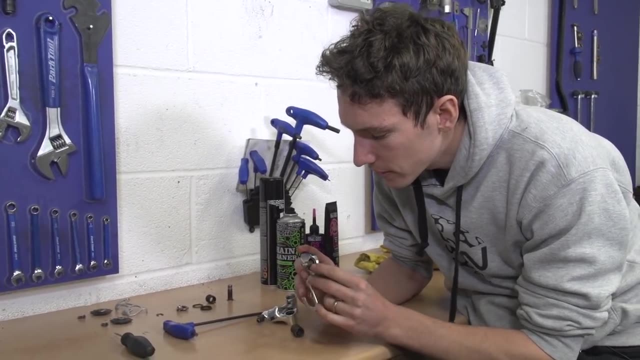 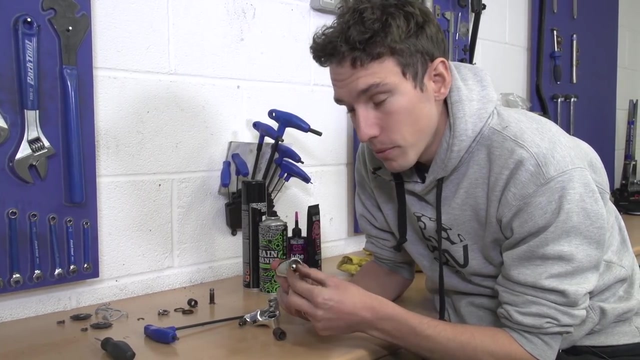 Can you see that, Okay, we are as clean as we're gonna get? and you can see, actually now, if you look closely, there is quite a bit of corrosion on the bushing there, so we maybe need just to take the very edge of that off. 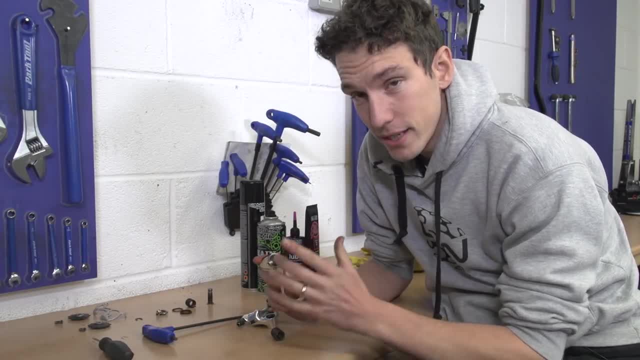 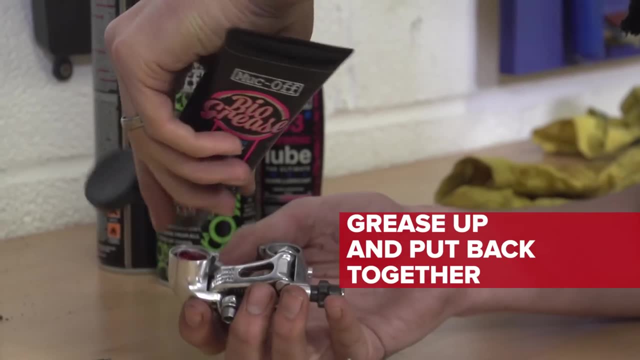 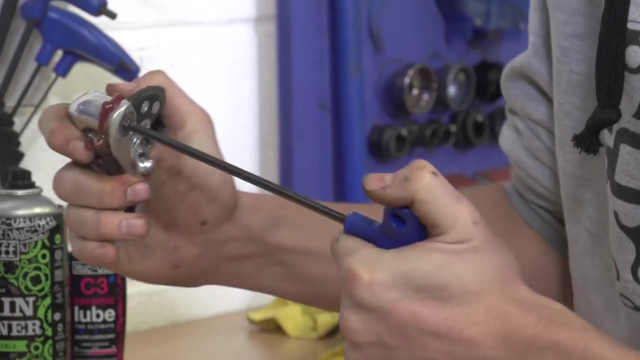 with a tiny bit of emery paper, but hopefully, hopefully, just a thorough re-grease is gonna get it back, so it is at least functioning again. Okay, there we go. Just functioning again. keep your fingers crossed. Ah, how satisfying is that. 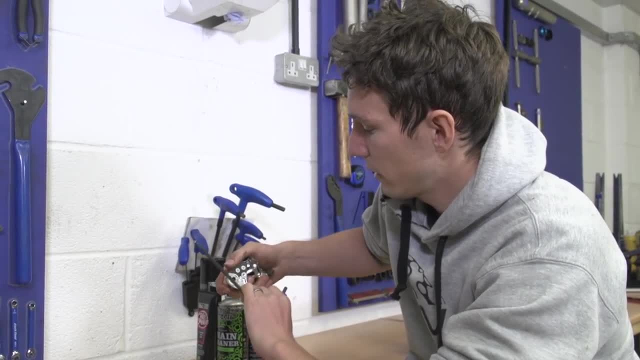 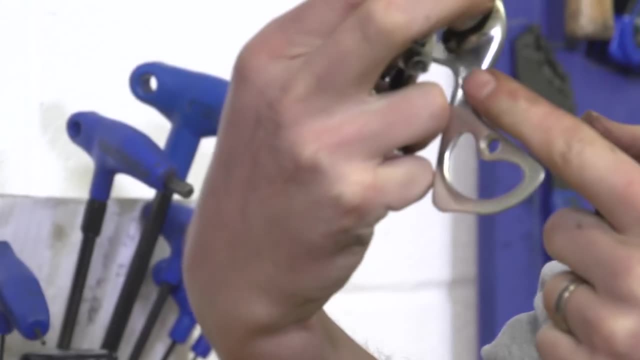 Now remember, as we're tightening that screw, we also need to move the lower cage of the rear derailleur so that it is in its normal place and if you remember, there was that stopper screw just on the back, so that needs to clear the derailleur cage. 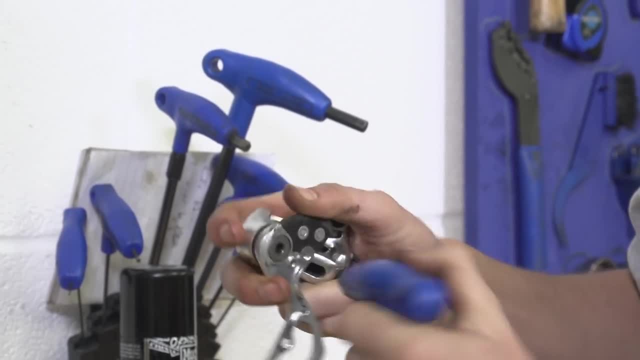 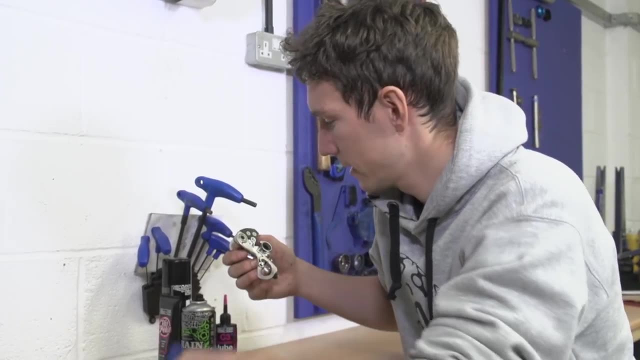 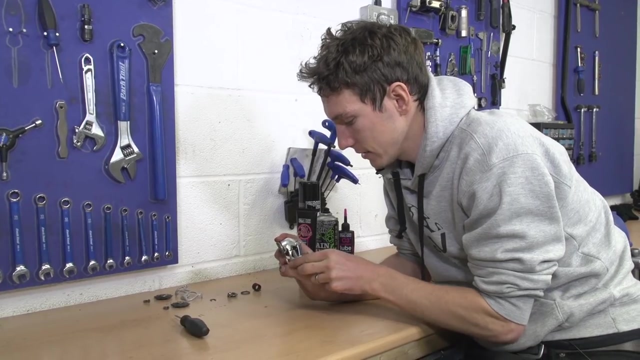 And then, as we tighten the screw, it holds it in place. So that is now back working. There we go. sneak preview: Look at that, I'm feeling good about this repair. Let's do the top pivot now. So that is all thoroughly cleaned. 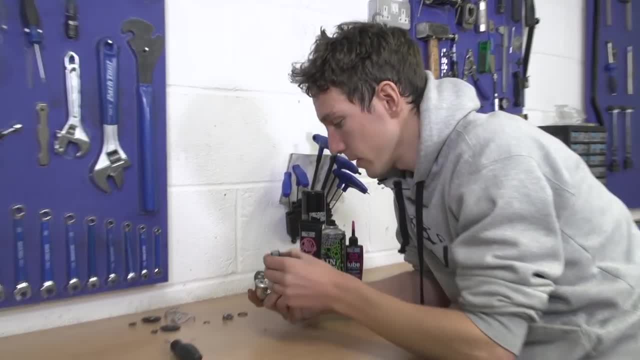 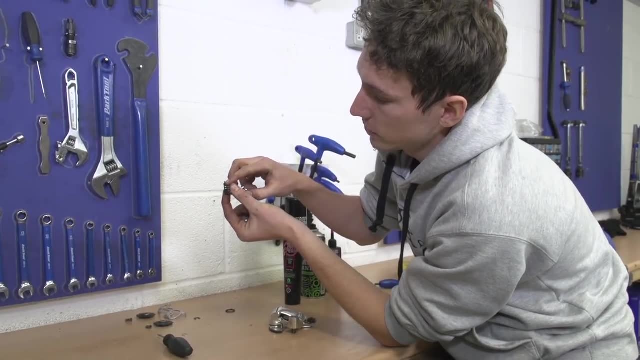 Push the pivot bolt back in. Then our spring. you can see the hole inside there. That's what we need to locate. Now, if you look at that spring, you'll see that it's not actually working. It's symmetrical. 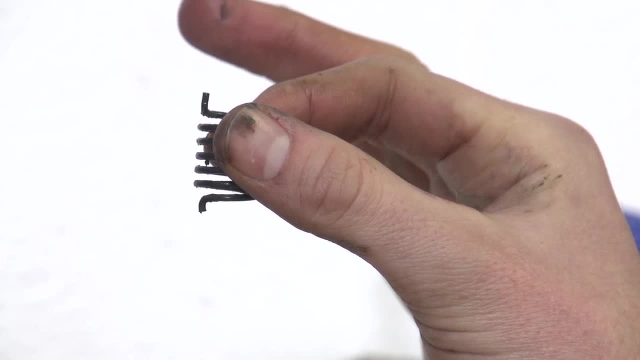 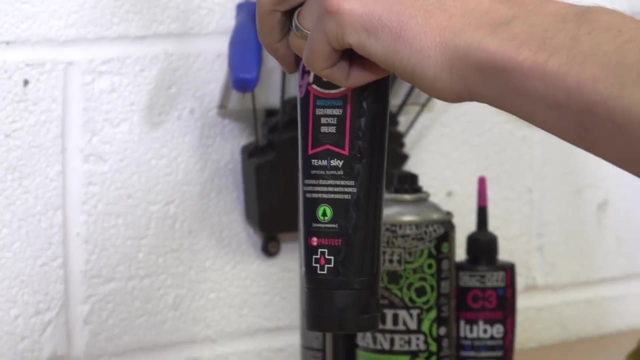 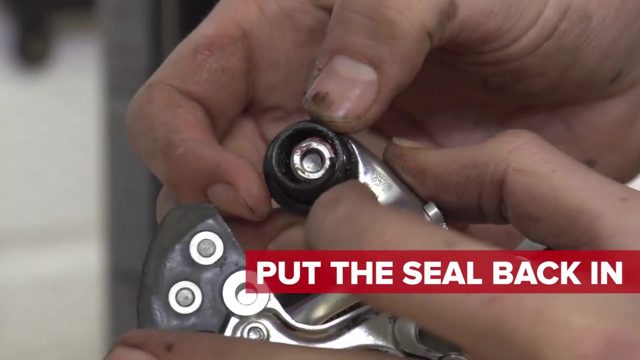 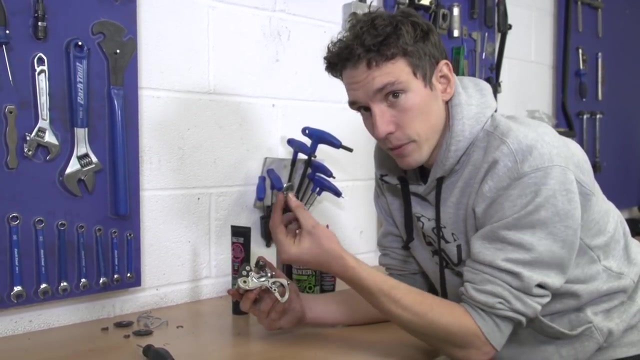 One little prong is longer than the other. So the longer prong goes inside the actual body of the derailleur itself, More grease. Then there we go. This last bit is going to be the trickiest bit. So we have to put our B-tension adjustment plate. 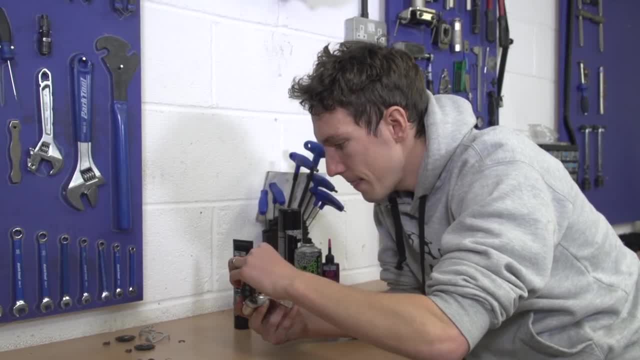 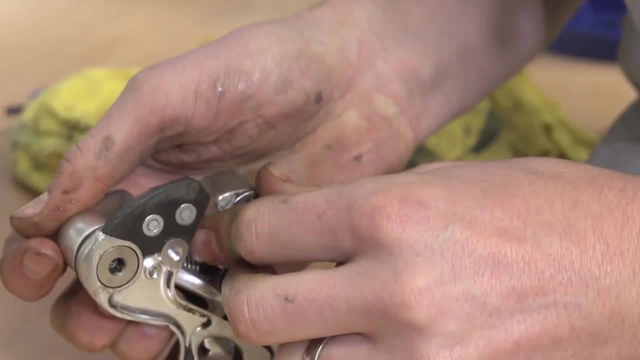 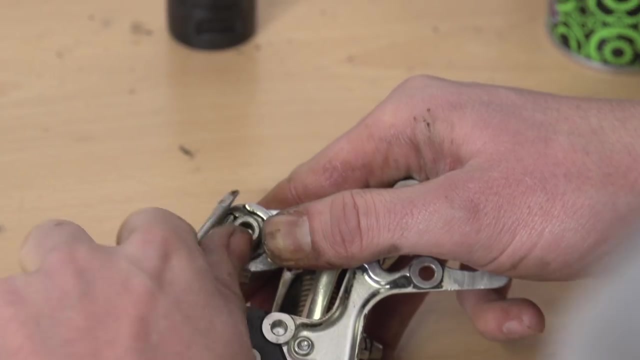 back over the spring. So we line it up And then we have to twist it counterclockwise to load the spring, whilst pushing it in, holding it in place and then grabbing our circlip there and pushing it back into place so that it all locks. 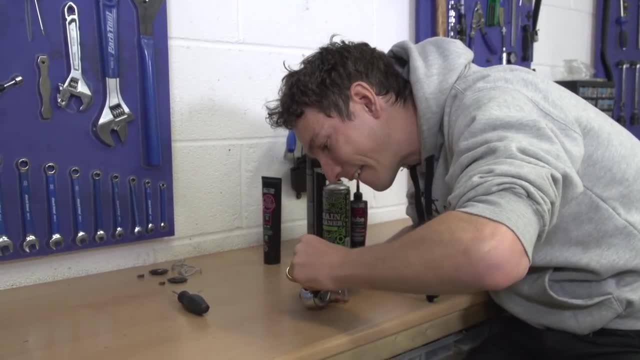 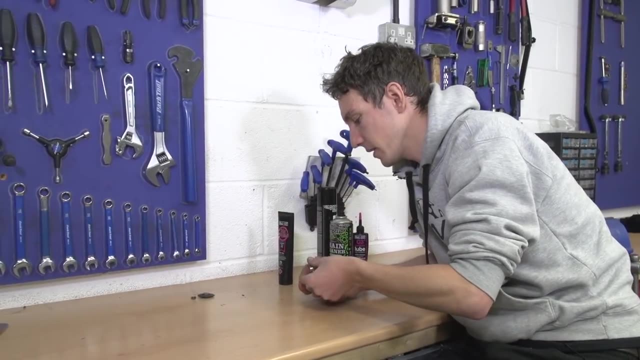 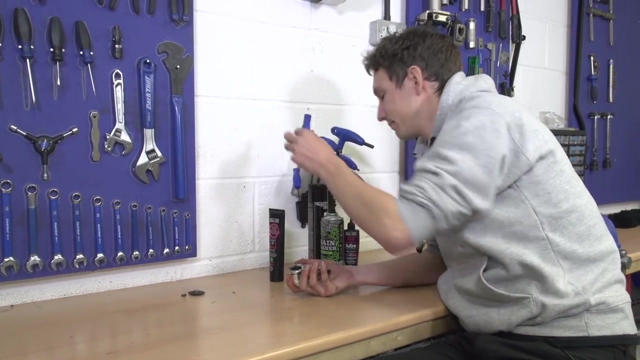 Ugh, come on, do it quick, quick, I'm in. We've just got to put our jockey wheels and cage back together now. I did say that this rear derailleur does need new jockey wheels, but for the sake of this, 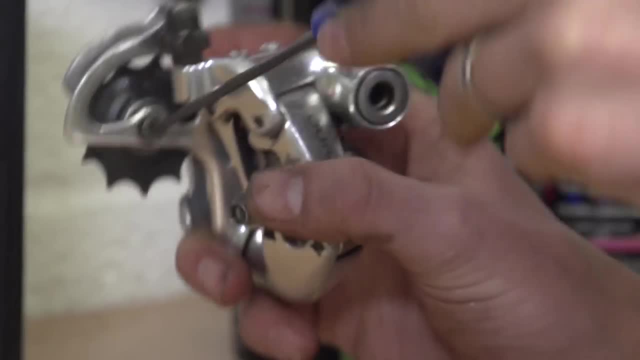 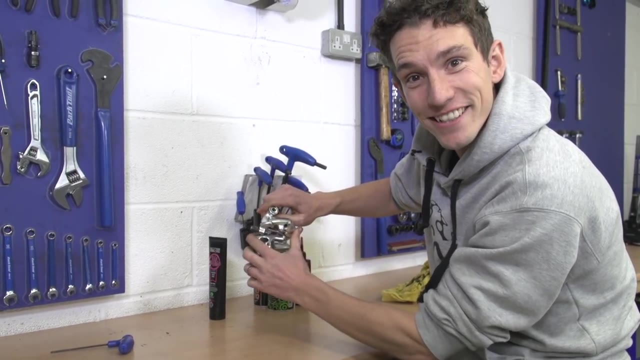 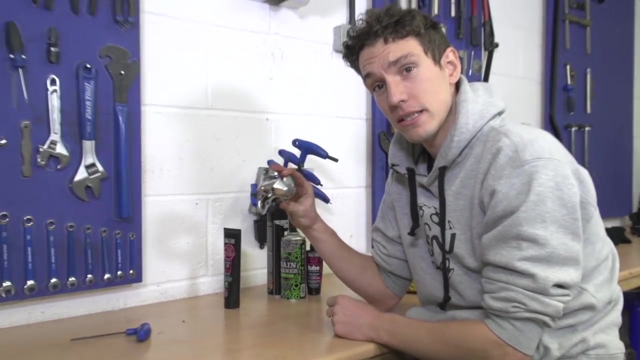 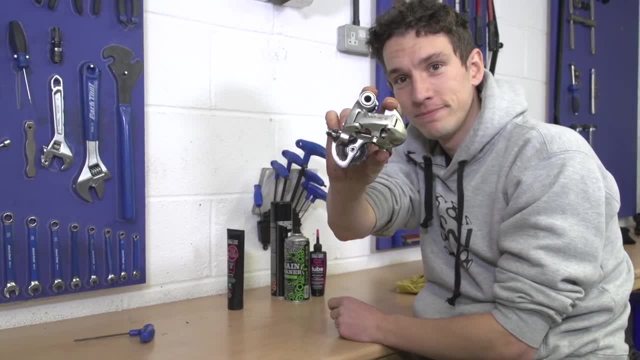 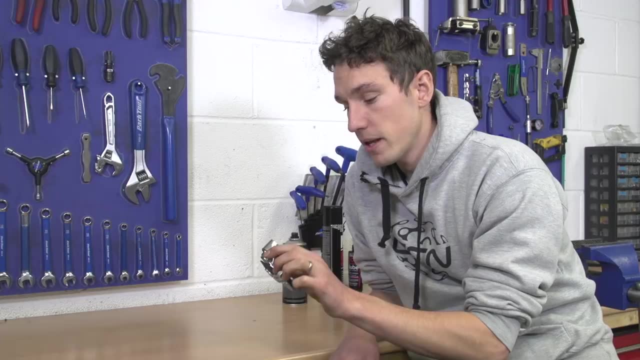 One successful renovation of a Shimano 7700RX. It's back in action. That's the method for a Shimano Dura-Ace 7700 rear derailleur. Most Shimano rear derailleurs are gonna be very similar to this. 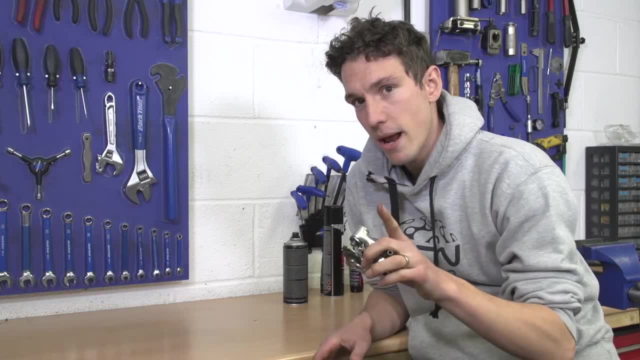 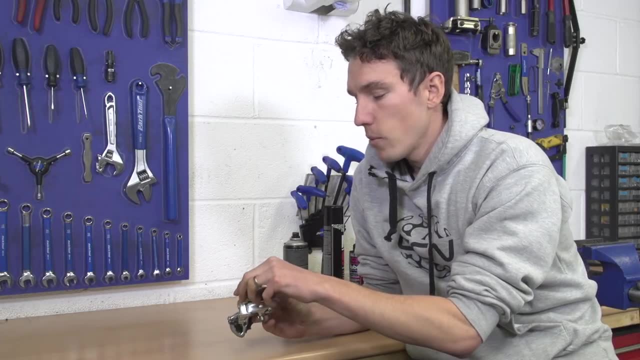 Most Campagnolo rear derailleurs will also be quite similar to this, but SRAM is slightly different. So that top pivot there that doesn't have a spring in it, so it won't ever freeze, but you will occasionally perhaps need to lubricate it. 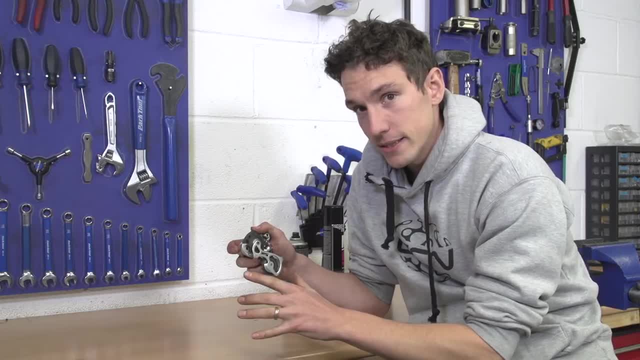 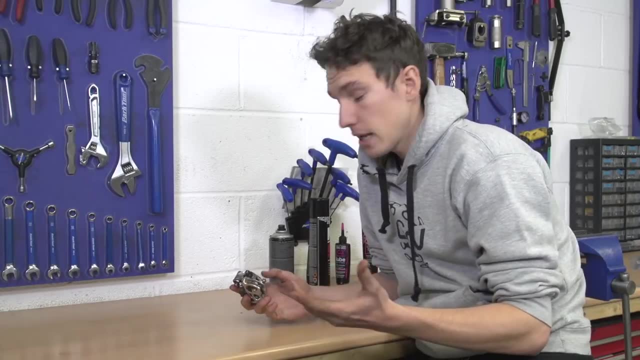 And then that lower pivot there That cannot be serviced. so do not try disassembling that, because you will come rapidly unstuck. Well, that hasn't really taken all that long, actually, to bring back what is rapidly becoming a piece of history to life. 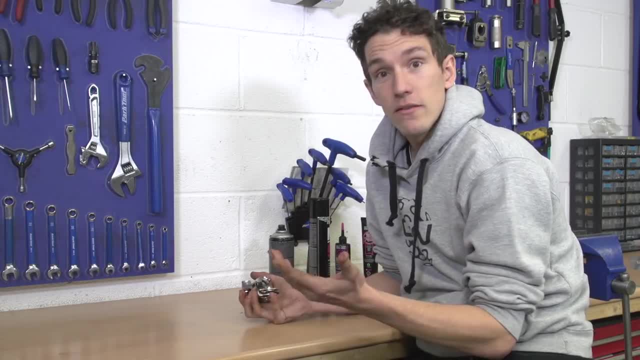 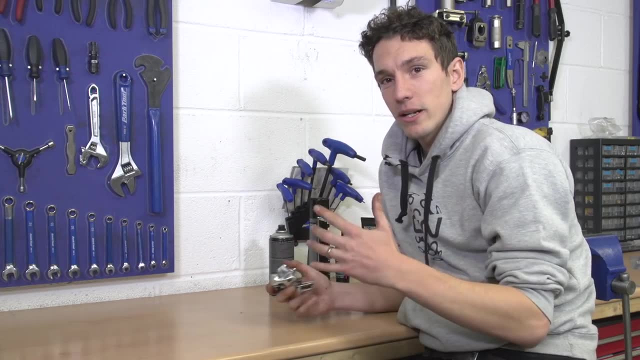 In fact, it's taken considerably less than an hour, so you don't even need all that much spare time. Just remember that when you do sit down to do a job like this, you've got a good place to do it, so that you're not gonna be losing.